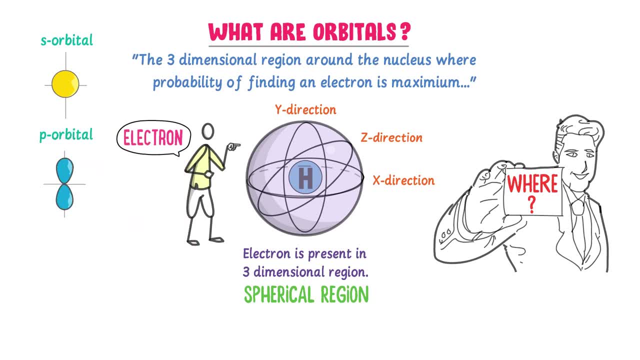 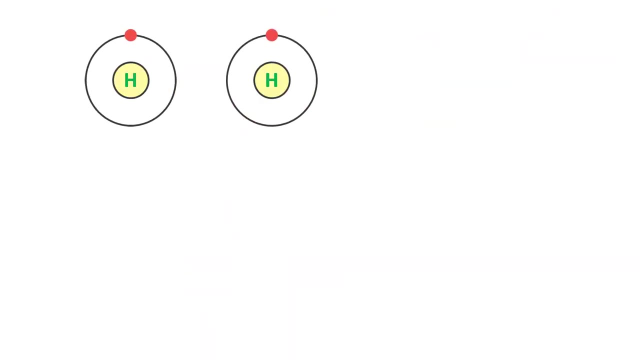 orbital is spherical, the shape of p orbital is dumbbell and the shape of d orbital is double dumbbell. Thus note it down that atomic orbitals are the three-dimensional region where we can locate electrons of any atom. Now let consider this hydrogen atom and this hydrogen atom. 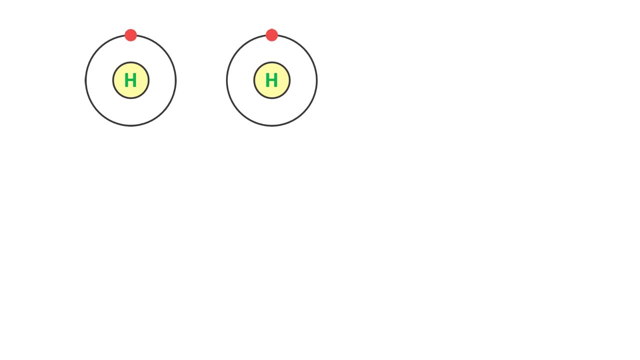 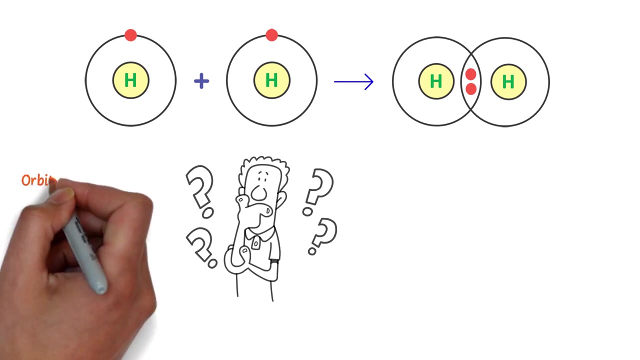 We know that each hydrogen atom has one electron. Now these two hydrogen atoms will react with each other to form a hydrogen molecule, H2.. Now here is the interesting part of the lecture. Have you ever wondered, or you ever asked your teacher, how the orbitals of hydrogen atoms combine together to form a hydrogen molecule? 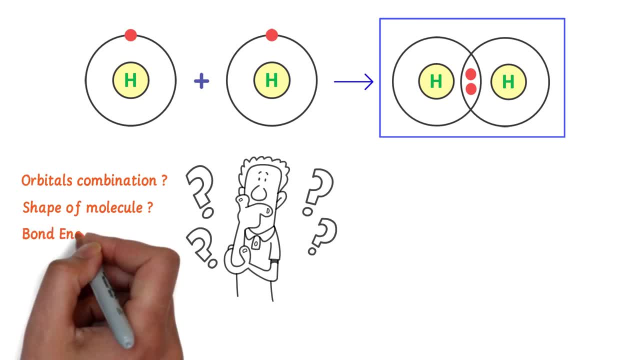 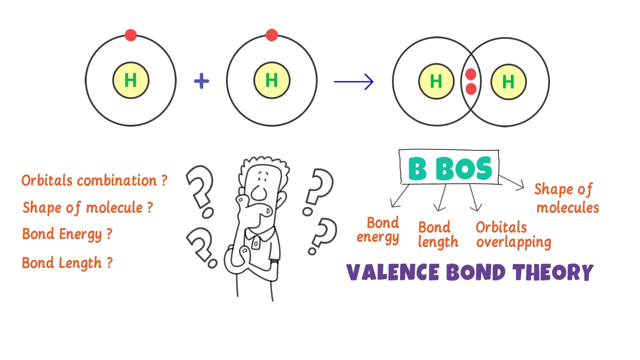 What about the shape of hydrogen molecule? What about the bond energy and bond length of a hydrogen molecule? Can you answer all these questions? Well, to learn about hydrogen molecules, we will use a combination of terazuga, and the answer is simple. 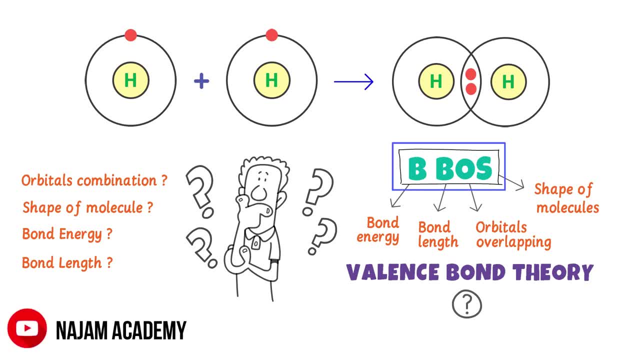 Valence Bond theory teaches us methane and dibergft. Valence Bond theory teaches us surround 않 Arrow and the alder garcias Calor. this energy is fouled and so it contains potassium, So it has back included hydrogen bond, energy, bond length, orbitals, overlapping and shape of a molecule. 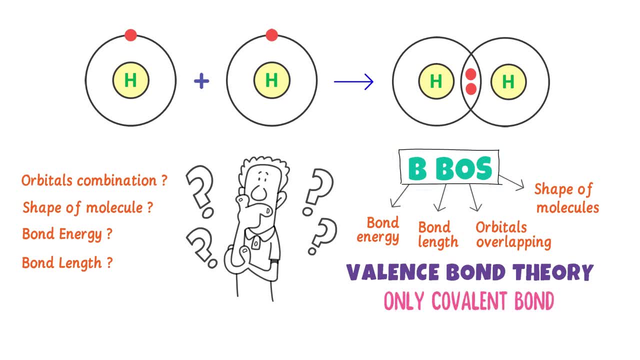 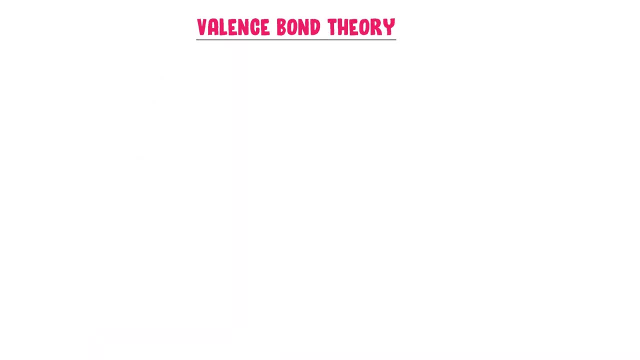 Also remember that VBT only explains the formation of a covalent bond. It does not explain ionic bond and metallic bond. Thus noted down all these important points. Now what are the postulates or key concepts of valence bond theory? Well, the first point of VBT is the formation of covalent bond. 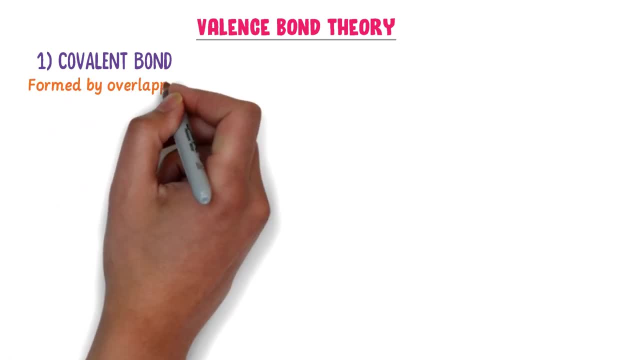 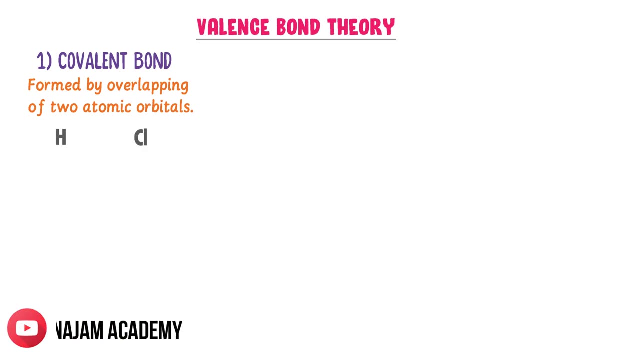 It states that covalent bond is formed by overlapping of atomic orbitals of two atoms. For example, consider hydrogen atom and chlorine atom. The last r-valence orbital of hydrogen atom is s-orbital and the last r-valence orbital of chlorine atom is p-orbital. 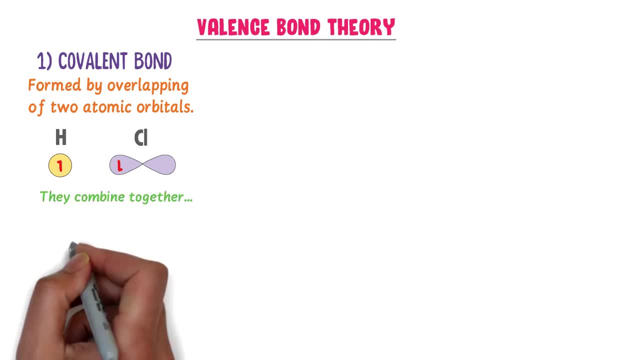 The valence orbitals of these both atoms will overlap together to share electrons and form HCl molecule. This region is called overlapping region, which has maximum density of electrons. Hence VBT teaches us that covalent bond is formed by overlapping of atomic orbitals. 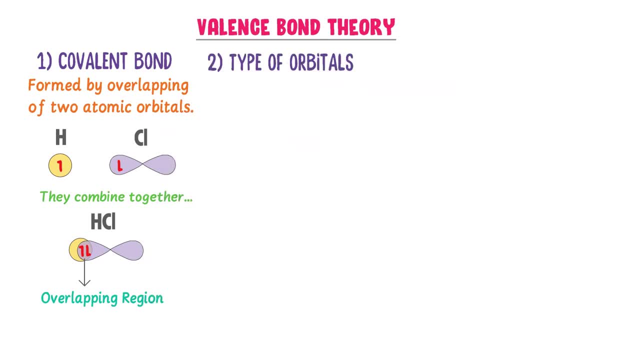 The second point of VBT is the type of orbitals. It teaches that only half-filled orbitals overlap to form a covalent bond. For example, in the case of HCl molecule, the s-orbital of the hydrogen atom has one electron. 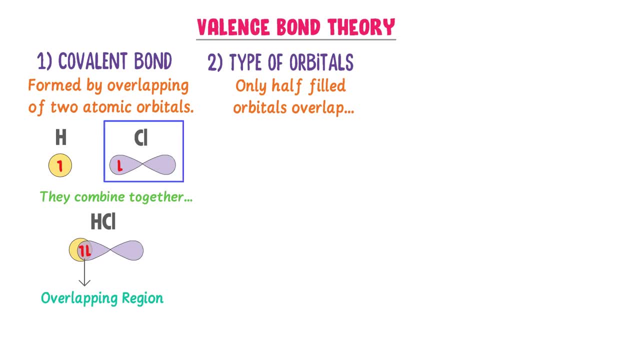 and two electrons, And the p-orbital of chlorine has one electron, So they both are half-filled. As a result of this, they overlap together to form a covalent bond and HCl molecule Also. let's consider this case. 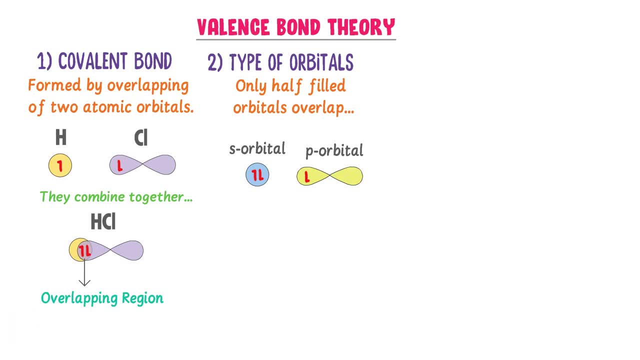 Here there are two electrons present in s-orbital, while one electron is present in p-orbital. The covalent bond does not form between them because s-orbital is complete having two electrons. Hence VBT teaches us that covalent bond is formed by overlapping of two electrons. 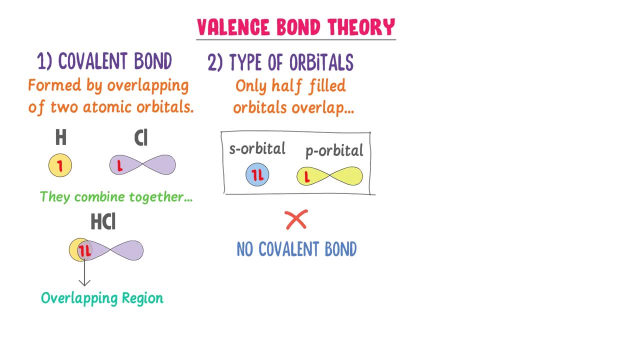 VBT teaches us that covalent bond is only formed if both the orbitals are half-filled, are having one electron each. The third point of VBT is the spin-off electron. It teaches that the spin-off electrons must be opposite and overlapping orbitals to form 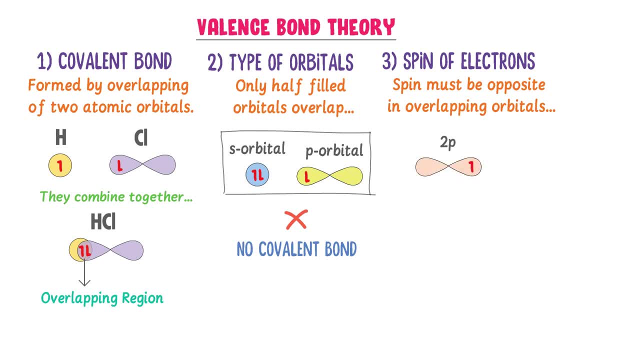 a covalent bond. For example, consider this case. Here the spin-off electron in 2p is upward, while that in 1s is downward. Hence these both orbitals will overlap together because they have opposite spin. Secondly, consider this case. in this case the spin of electrons in either orbital is: 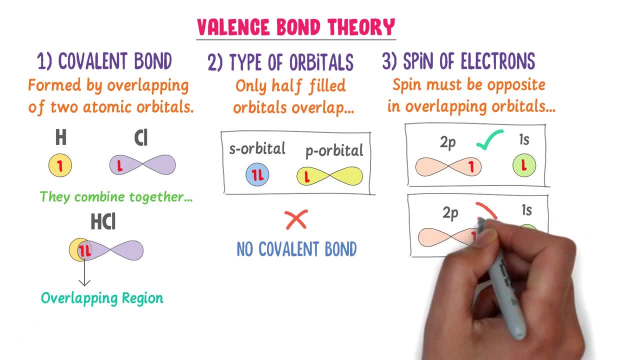 upward. they will not overlap together because they have the same spin. Thirdly, consider this case. in this case, one orbital is completely filled. we need both orbitals to be half filled so they will not overlap together to form a covalent bond. 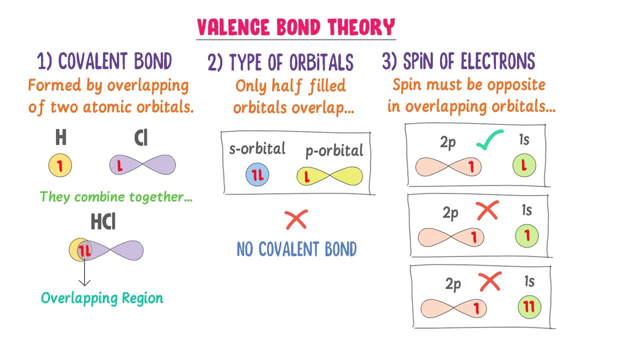 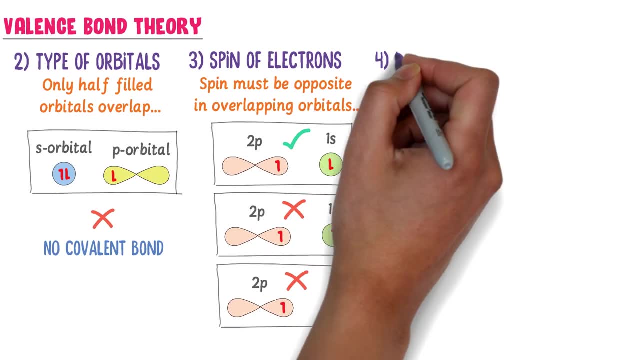 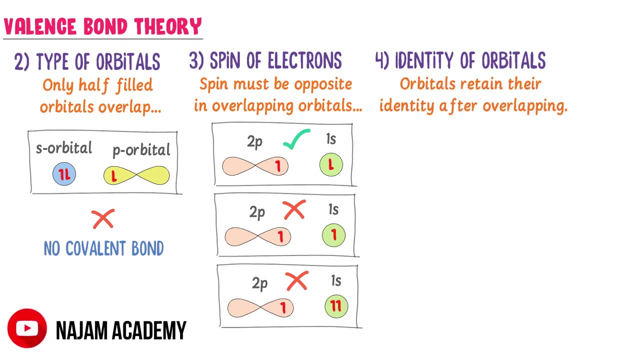 Thus, VBT teaches us, the spin of electrons must be opposite in orbitals to overlap and form a covalent bond. The fourth point of VBT is the identity of orbitals. It teaches that orbitals retain their original identity after overlapping. 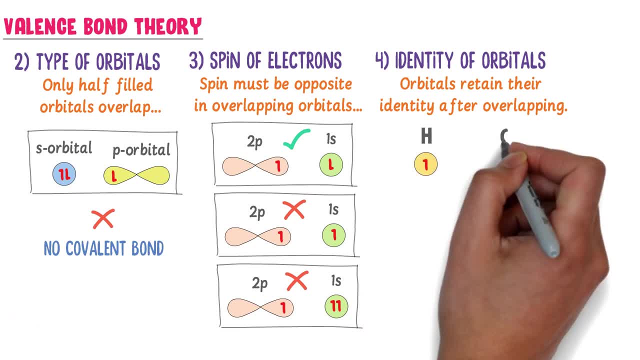 For example, consider the s-orbital of hydrogen and p-orbital of hydrogen. The ship of s-orbital is spherical and that of p-orbital is dumbbell. When hydrogen atom and chlorine atom react to form HCl, still the atomic orbital of hydrogen. 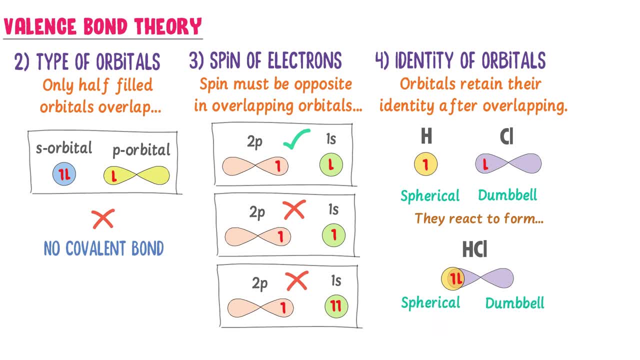 is spherical and that of p-orbital is dumbbell. It means that they both have retained their original shape or original identity. But remember that the energy of atomic orbitals is high before overlapping. Once they overlap, then they have lower energy and a molecule. 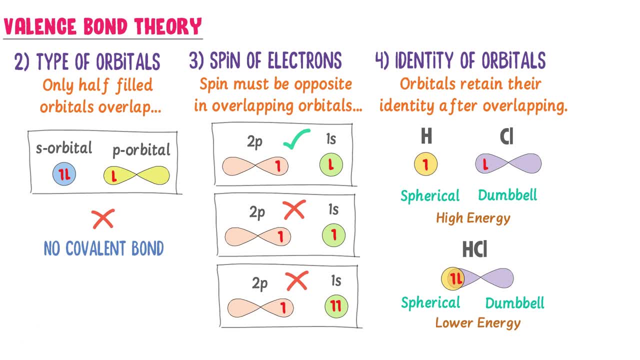 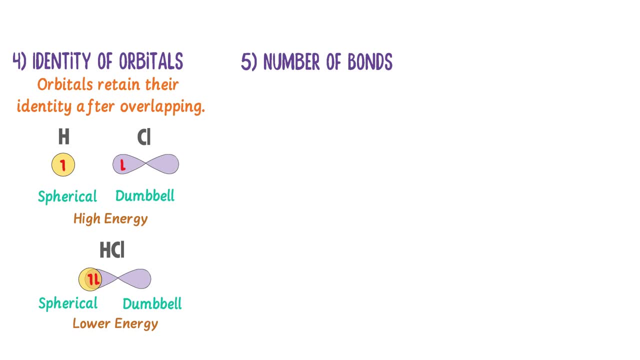 Thus, VBT teaches us that orbitals retain their identity after overlapping. The fifth point of VBT is number of bonds. It teaches us that if there is 1 unpaired electron, it will form 1 covalent bond. If there are 2 unpaired electrons, it will form 2 covalent bonds. If there are 3 unpaired bonds, it will form 3 covalent bonds, And if there are four unpaired electrons, it will form four covalent bonds. For example, in case of nitrogen, there are three unpaired electrons present in each orbital. 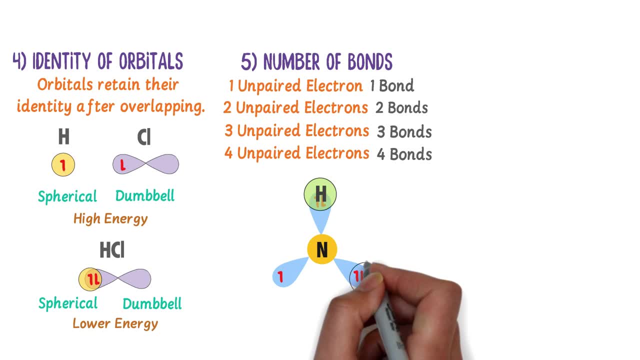 Hence nitrogen atom share its three unpaired electrons with one electron each of three hydrogen atoms to form NH3 or ammonia. So due to three unpaired electrons, nitrogen atom forms three covalent bonds. Thus VBT teaches us the number of bonds. 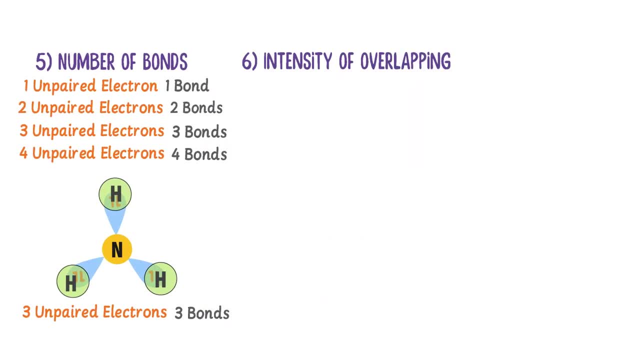 The sixth point of VBT is the intensity of overlapping. It teaches that overlapping between orbitals should take place at optimum or suitable position. For example, consider overlapping of two atomic orbitals of A and B atoms. In this case, the atomic orbitals overlap. 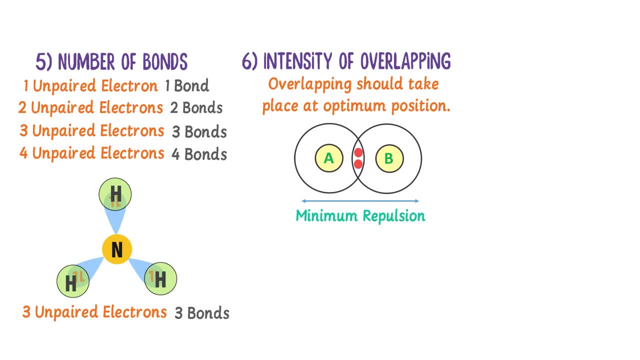 in the same way, At such a position that the repulsion between the two nuclei is minimum. So we say that overlapping between orbitals take place at optimum or suitable position, While in this case the two atomic orbitals overlap so close that the two nuclei can almost 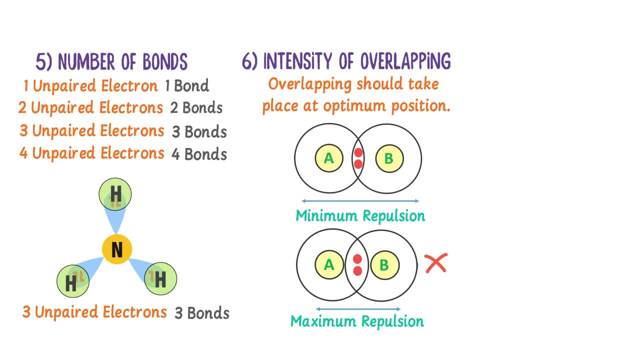 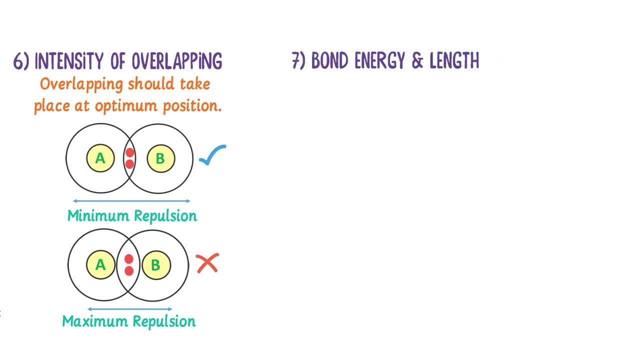 touch each other. So this is the wrong case of overlapping and it will not happen While this is the right case. Thus, VBT teaches us the intensity of overlapping. The 7th point of VBT is bond energy and bond length. It teaches that the extent of overlapping decides the bond energy, bond strength or 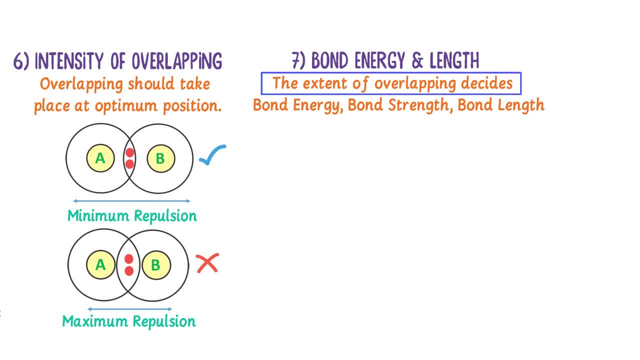 bond length. We can say that the extent of overlapping is directly proportional to the bond energy or bond strength. If overlapping is greater, bond strength or bond energy would be high. For example, consider overlapping between these two P orbitals. Let there is minimum overlapping between the two orbitals. 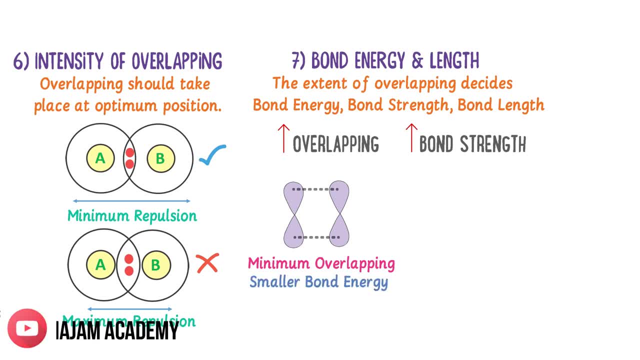 So the bond energy will be smaller. Secondly, minimum overlapping means that the two orbitals will be away from each other, So the bond length will be high. Now consider overlapping between these two orbitals. Let there is maximum overlapping between them, So the bond energy or bond strength will be high. 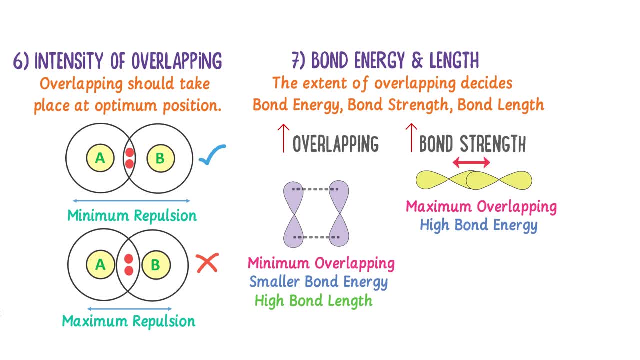 Secondly, maximum overlapping means that the two orbitals will be close to each other, So the bond length will be smaller. Hence noted down that if the overlapping is minimum, bond strength or bond energy will be smaller and bond length will be high. If the overlapping is maximum, bond strength or bond energy will be high and bond length 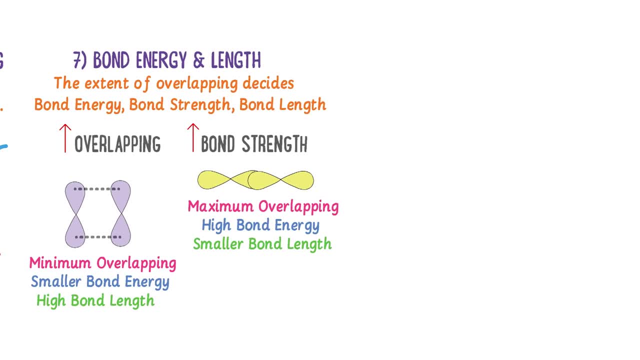 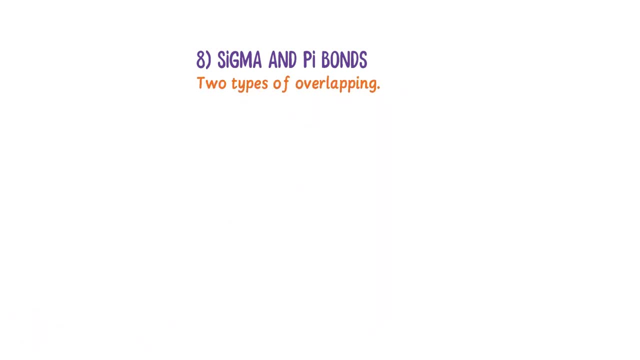 will be smaller. The last and add point of VBT is the sigma and pi-bar. It teaches that there are two types of overlapping occur between atomic orbitals: Axial overlapping, which is also known as head-to-head overlapping, and parallel overlapping, which is also known as side-to-side overlapping. 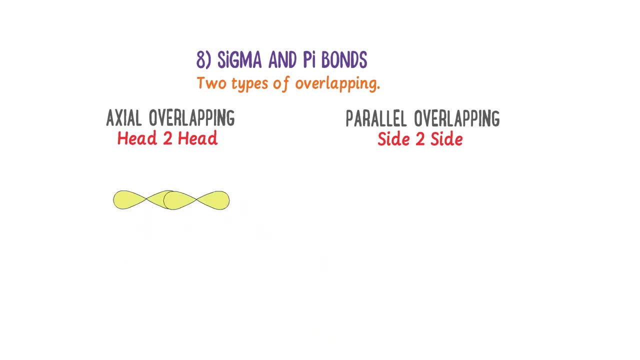 For example, when two p orbitals overlap like this, it is called axial overlapping or head-to-head overlapping. Remember that This type of overlapping will also occur when two p orbitals overlap like this. Remember that This type of overlapping will also occur when two p orbitals overlap like this: